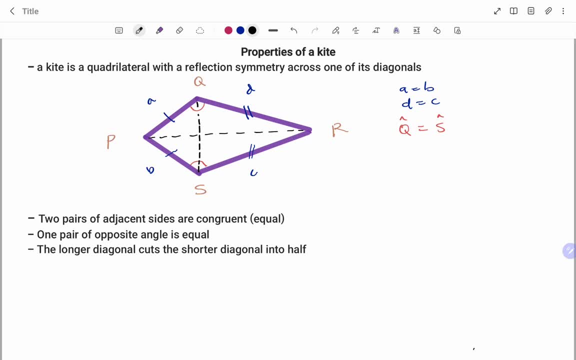 one says the longer diagonal cuts the shorter diagonal into half. PR is the longer diagonal. That means it cuts or bisects QS. So this line is equal to the first line. Let me call this point where they meet point T. So that means QT, QT, the. 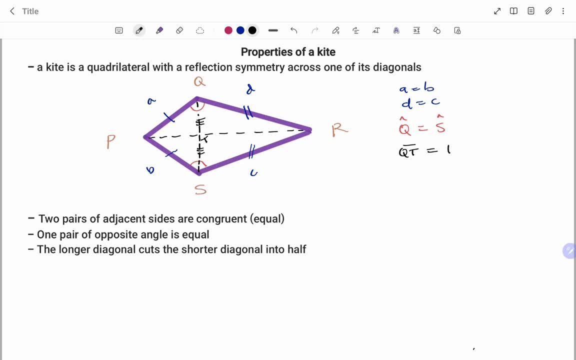 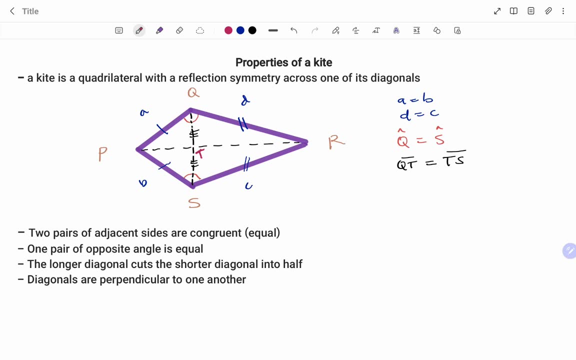 line QT is equal to the line TS. The next property states that the diagonals are perpendicular to one another. So the diagonals PR and QS are perpendicular. So I'm going to put symbol right here. That means the line PR is perpendicular to the line QS. The last but not the least, 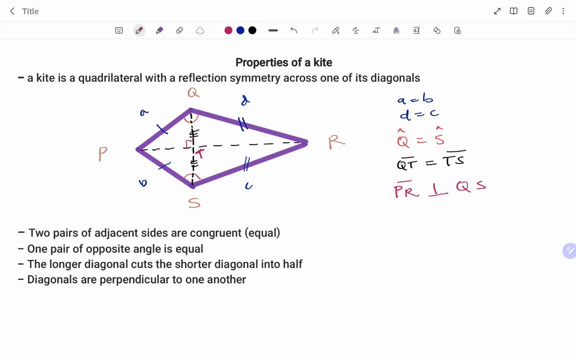 property states that the longer diagonal, which is PR, as SHUN, bisects the angles. So therefore, this angle is equal to this angle. Likewise, this angle is equal to this angle. So go, the side A is equal to the side B, as shown, and the side D is equal to the side C. Then, 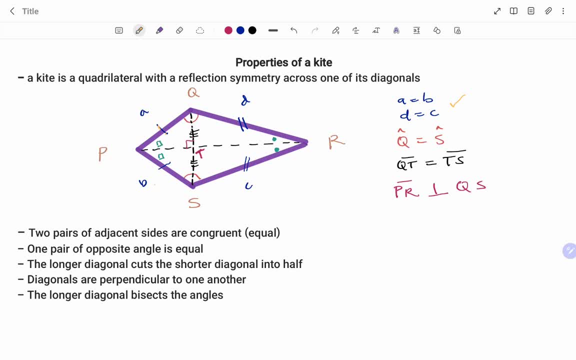 one pair of opposite angle is equal. Angle Q is equal to angle S. The diagonal cuts the shorter diagonal into half. Yeah Yeah, The longer diagonal is your PQ and the shorter diagonal is your QS. The diagonals are perpendicular to one another. therefore, PR is perpendicular to QS. 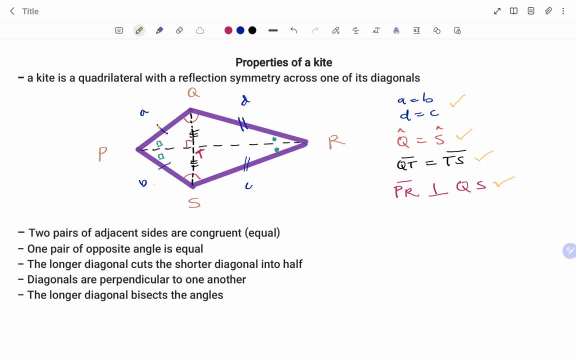 And the last property, but not the least, the longer diagonal bisects. the angle R1 is equal to R2 and P1 is equal to angle P2.. Thanks for watching. bye.